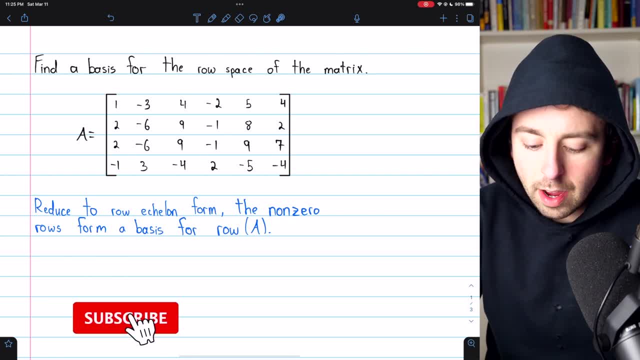 We're going to find a basis for the row space of this matrix. That means we're looking for a set of linearly independent vectors that span the row space. That's a basis. This is pretty straightforward. All we need to do is take this matrix A and reduce it to row echelon form. Then 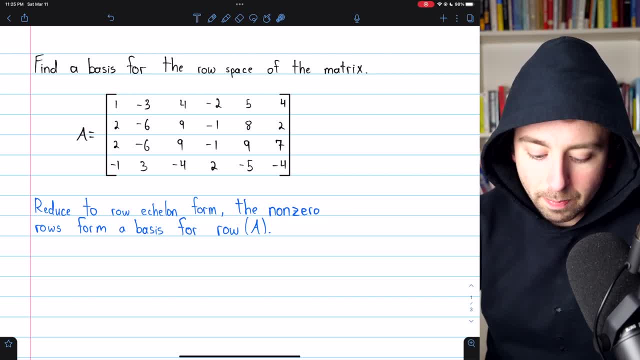 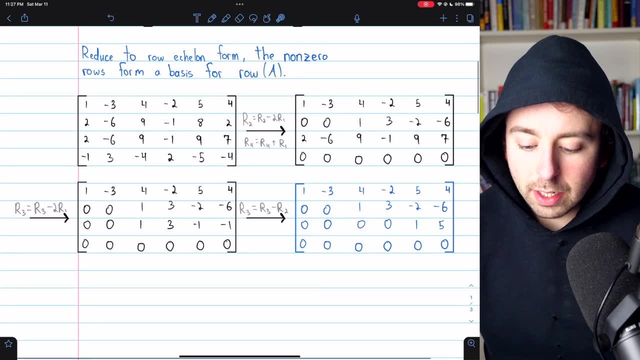 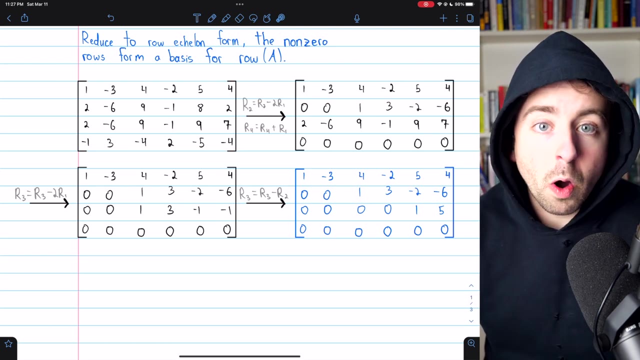 the non-zero rows in that echelon form will form a basis for the row space. I won't explain these elementary row operations in detail because you should be pretty familiar with the process. but this is the beginning. matrix A: Then here are the steps we take: the elementary row operations: 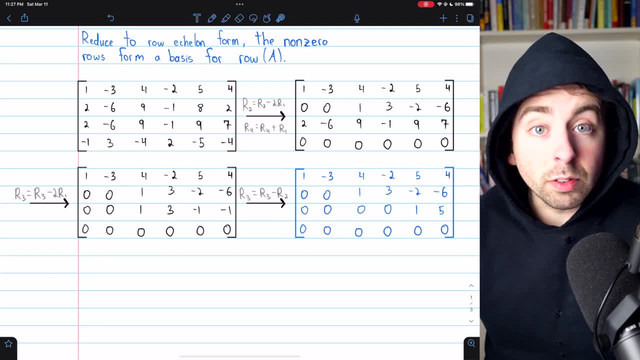 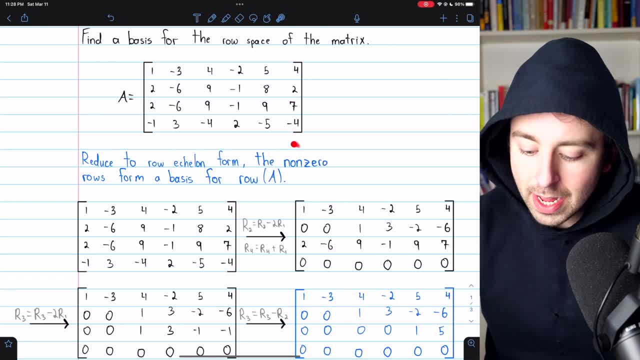 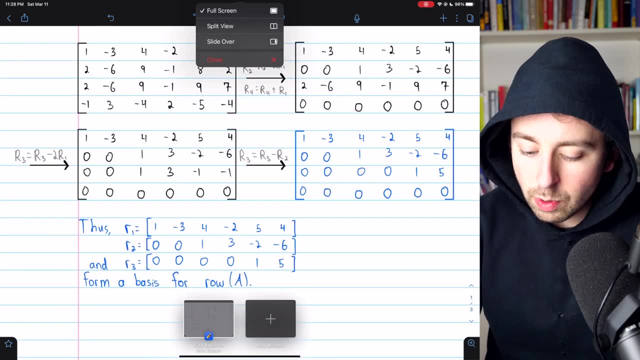 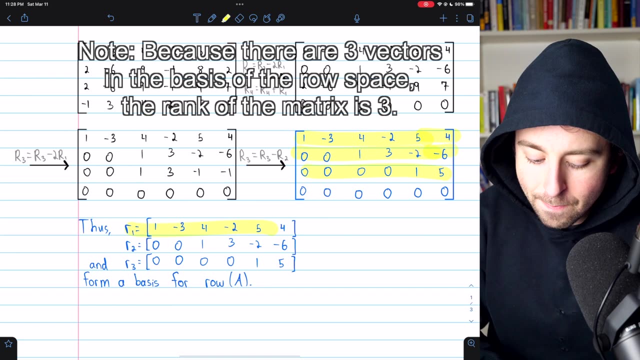 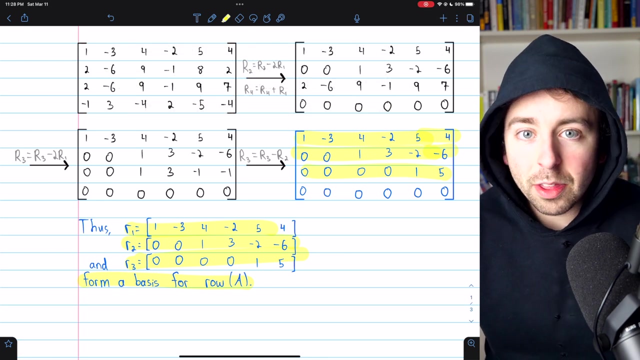 here. Remember, once we get our matrix in row echelon form, the non-zero rows form a basis for our row space. So we're pretty much done. We see, we've got these three non-zero rows and those three row vectors form a basis for our row space. So these are three linearly independent vectors that together span the row space. 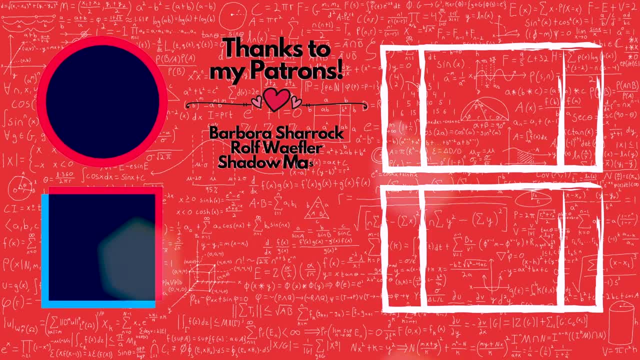